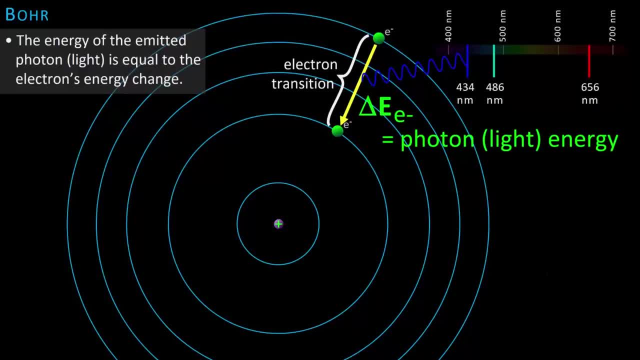 is equal to the electron's change in energy. The electron transitions from a higher to a lower energy and the difference is equal to the light energy emitted. This model of the atom came out of Bohr trying to figure out why various elements and compounds emit very specific frequencies of light. 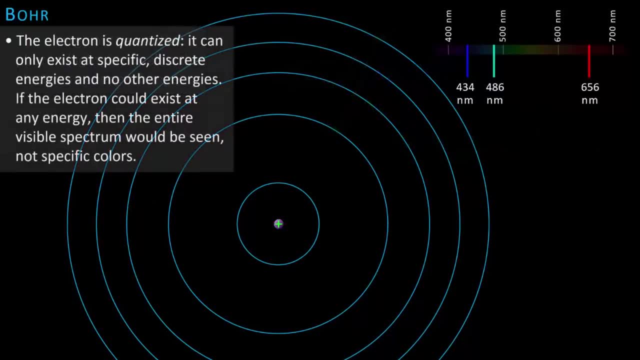 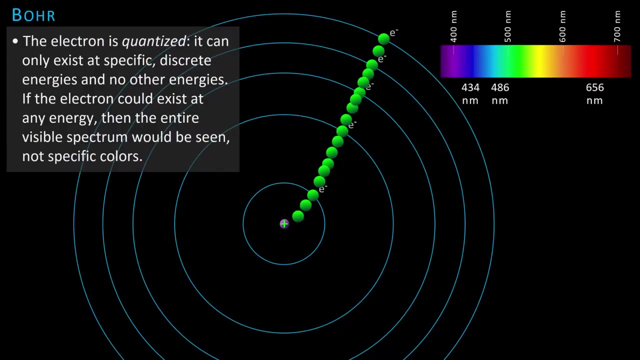 something that had puzzled scientists for decades. What is crucial here is Bohr's contention that the electron could only exist at discrete energies. In other words, the electron is quantized. If the electron could exist at any energy, then light could be generated at any energy due to the electron energy transitions occurring at any energy rather than discrete energies. 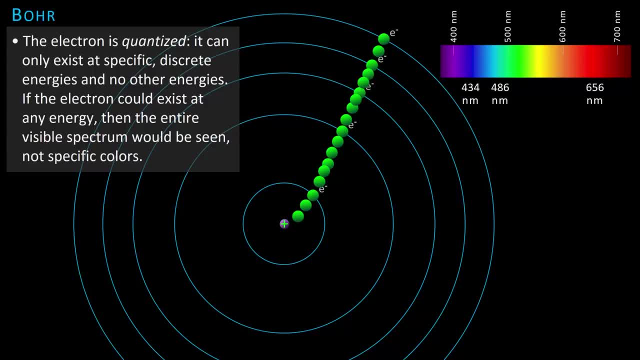 which we would observe as an entire rainbow of colors emitted rather than discrete individual colors. We don't observe a rainbow. We do observe discrete colors, and so the electrons can only transition between specific orbits, and therefore electrons can only exist at those energies. 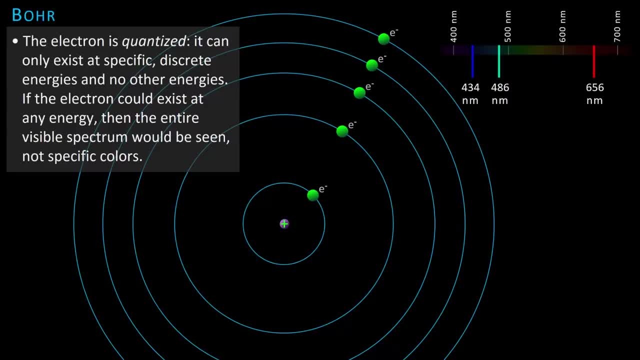 They cannot exist at energies in between. However, Bohr had no explanation for how the electron could exist like this in what is called a quantized state, where electron energy is discrete. Bohr's idea was a remarkable application of Planck's and Einstein's work. 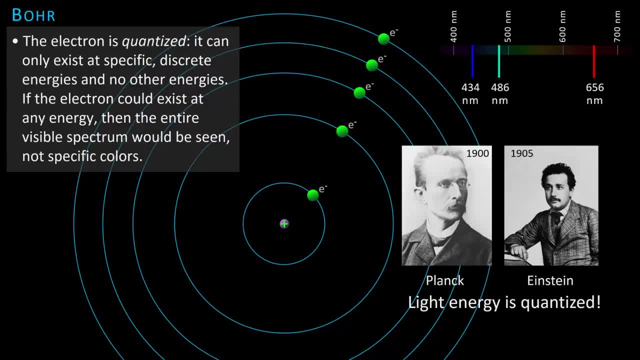 showing that light energy is quantized, But light has no mass. However, Bohr was quantizing a particle with mass, the electron. So now we can look at de Broglie's model as an explanation of Bohr's description of the electron as being quantized. 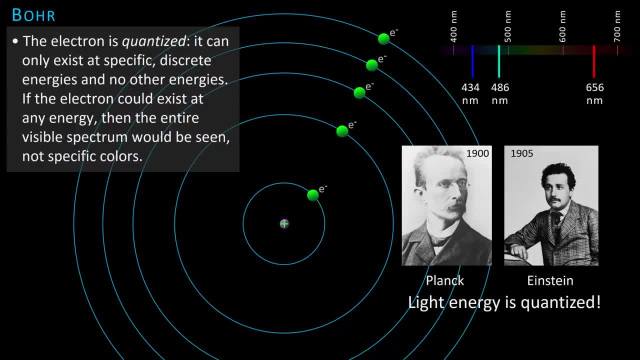 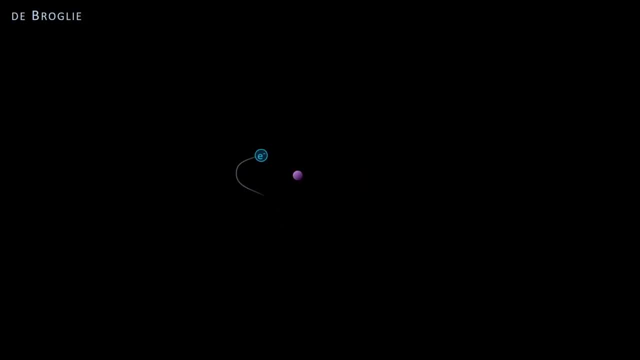 electrons only existing at specific discrete energies. So Bohr's model of orbits was supplanted by de Broglie's model of the electron traveling as a wave. What is important to understand about this wave behavior is that the electron is in phase with itself. 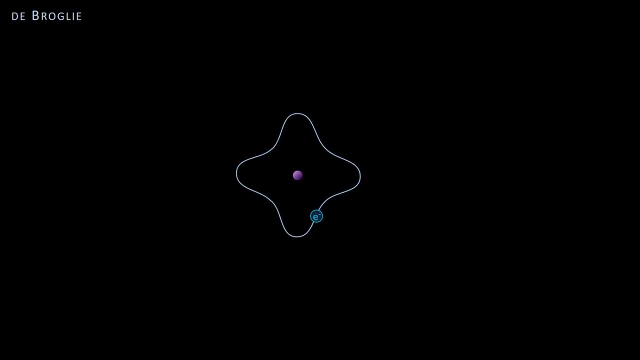 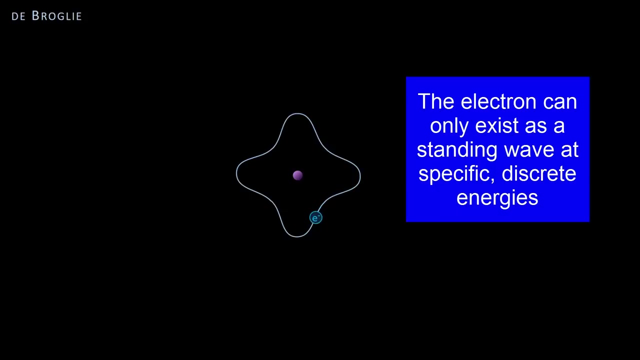 It meets its own path as it travels around the nucleus. This is called a standing wave, And the electron can only exist as a standing wave at specific, discrete energies. This is a commonly known function of standing waves. Here we have a path with four waves. 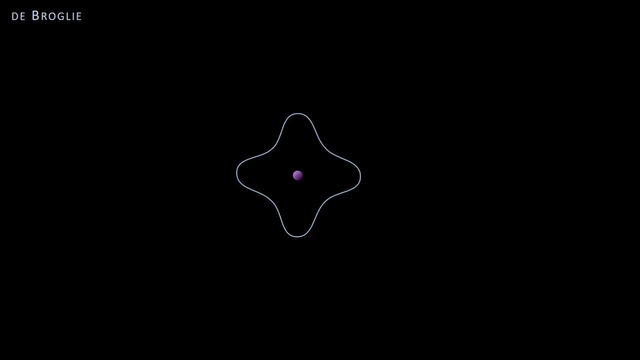 What would happen if the electron went to a higher energy level, Let's say from a path with four waves to a path with five waves. The standing wave with five waves would have to increase in size to accommodate the fifth wave, and so this higher energy path is larger. 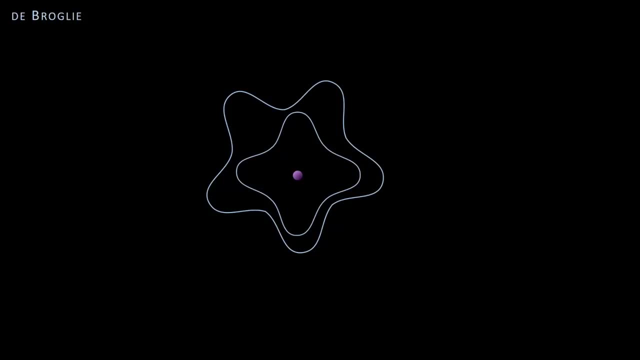 and so this higher energy electron is therefore further from the nucleus. This is what Bohr had stated with his circular orbit model, but without explanation. Here the size of the path would have to increase exactly to the point where another wave could fit into it. 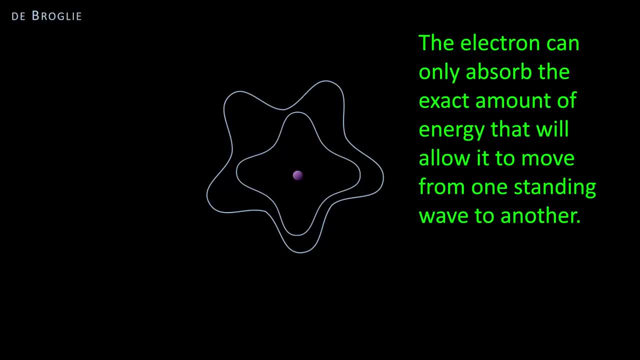 And so the electron can only absorb the exact amount of energy that will allow it to move from one standing wave to another. Bohr's quantized electron now makes sense. Let's enlarge the new standing wave for the sake of clarity. So 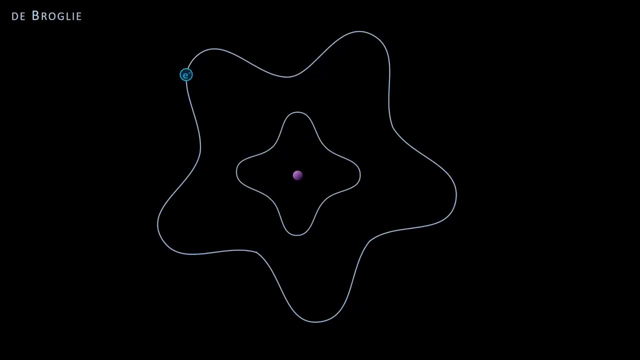 if the electron has gained the exact energy needed to go from a standing wave of four waves to five waves, it will exist at a standing wave of five waves. This brings up the question: what if it absorbs some amount of energy that is not enough to get it to a standing wave? 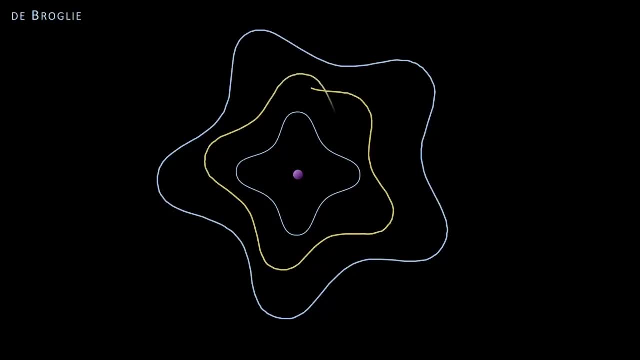 Let's see what would happen. The electron would not be in phase with itself, It would not exist as a standing wave. The electron would interfere with itself and could not exist on a path that was not in phase, a path that interferes with itself. 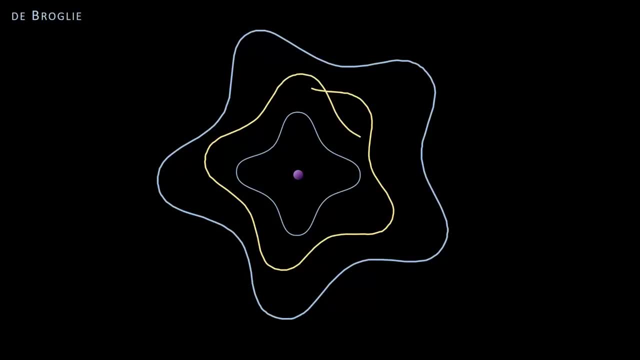 This is a beautiful explanation of Bohr's quantized electron. A very important part of Bohr's model is that if the right amount of energy is absorbed by the electron, it can then go to a higher energy orbit. Here the energy of red light is absorbed by the electron. 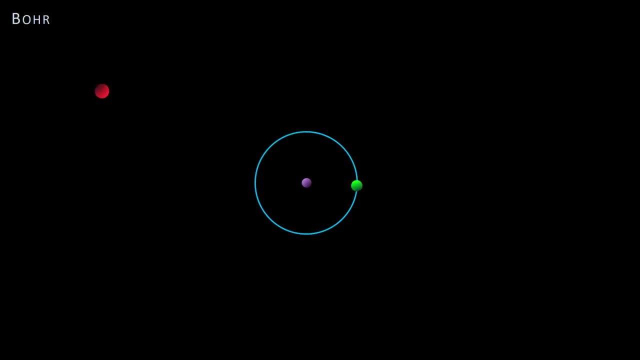 which pushes it to a higher energy wave, but it will want to get rid of excess energy and does so with the release of red light, while going back to a lower energy orbit. This explains the specific, discrete colors coming out of energized elements. For de Broglie, 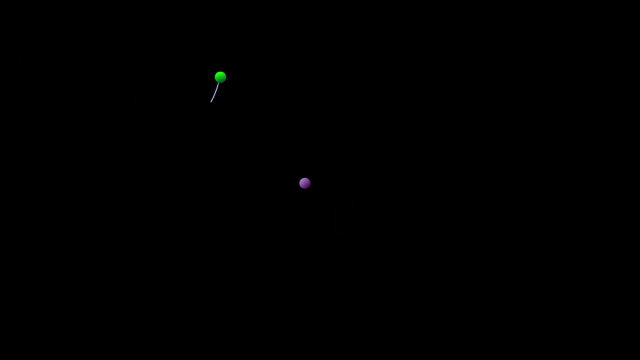 if the right amount of energy is absorbed by the electron, it can then go to a higher energy standing wave. Here the energy of red light is absorbed by the electron, which pushes it to a higher energy standing wave, but it will want to get rid of excess energy. 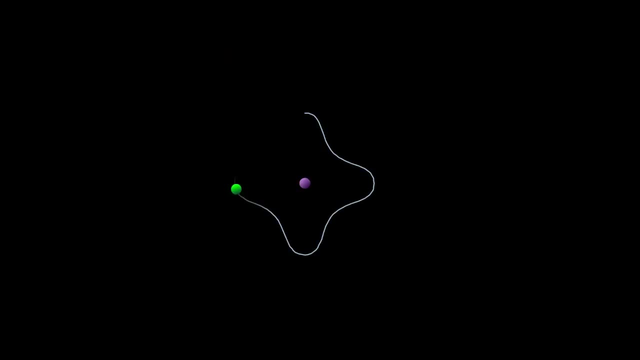 and does so with the release of red light, while going back to a lower energy standing wave. The electron cannot absorb any other energy, for example yellow or blue, because those colors do not have the energy required to get the electron to another standing wave. 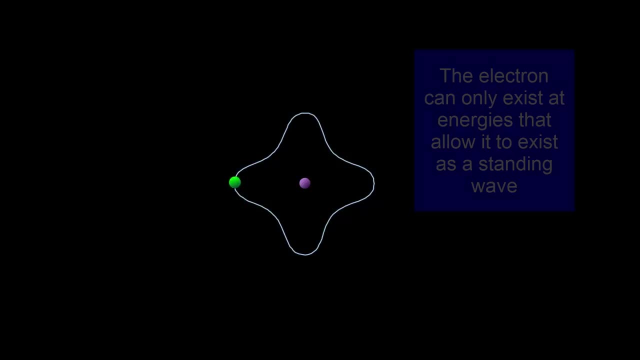 This explains the discrete colors coming out of energized elements. Bohr was correct in his remarkable application of quantized light to a quantized electron, which was subsequently shown to be correct through de Broglie and the current quantum mechanical model and many, many experiments confirming. 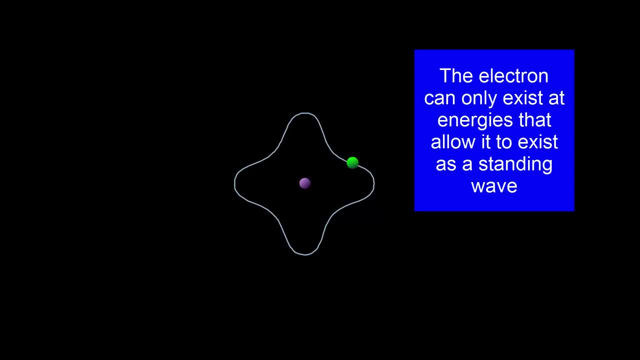 that electron energy is not continuous, but discrete. The electron can only exist at allowed energies, and so we say: the electron energy is quantized. So de Broglie succeeded in describing a mechanism, in Bohr's hypothesis, of quantizing electrons only existing at allowed energies. 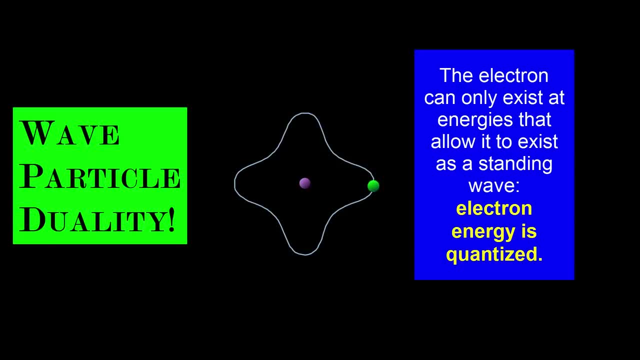 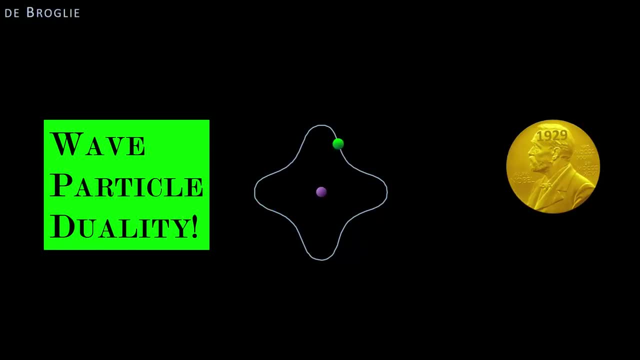 This established the wave-particle duality of matter, a monumental step in our current view of the universe. It earned de Broglie the Nobel Prize in Physics in 1929, only five years after its publication as part of his PhD thesis. 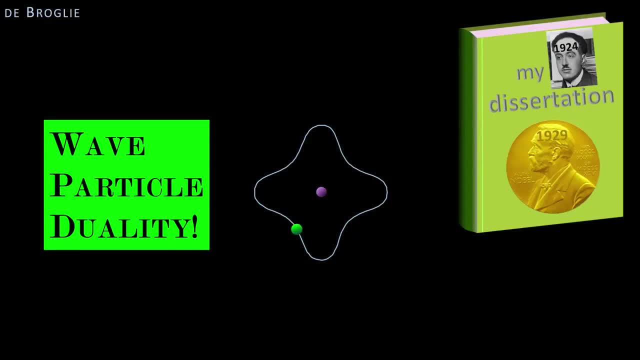 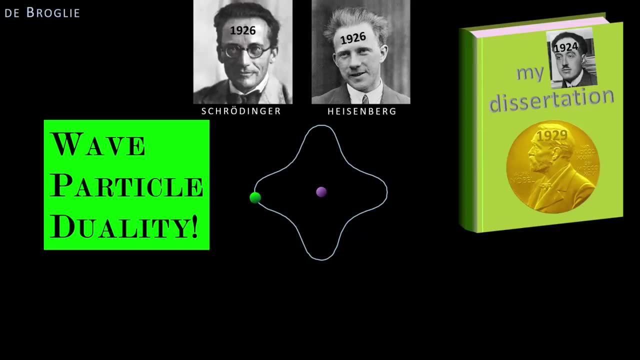 and was a critical step in establishing the quantum mechanical model of the atom two years later by Schrödinger and Heisenberg, a model which is intimately based on the wave properties of the electron devised by de Broglie. The electron's wave property presented in this video. 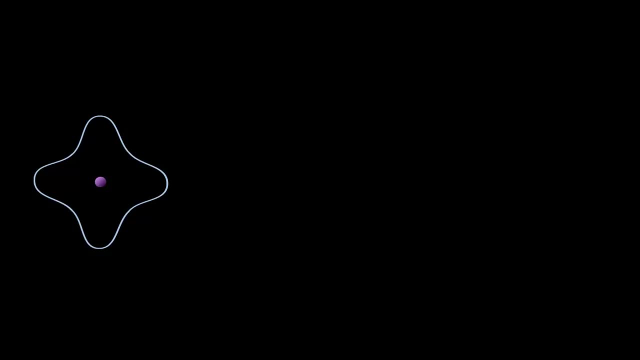 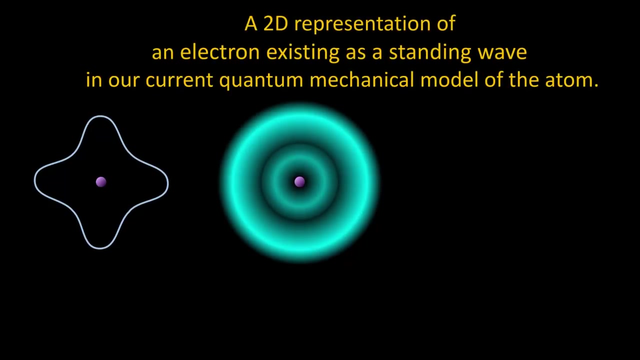 was de Broglie's interpretation of the mathematics he established to describe this wave-particle duality of the electron. but it is in fact very different from the now more established interpretation of the electron as wave. In 1926, Max Born interpreted the standing wave. 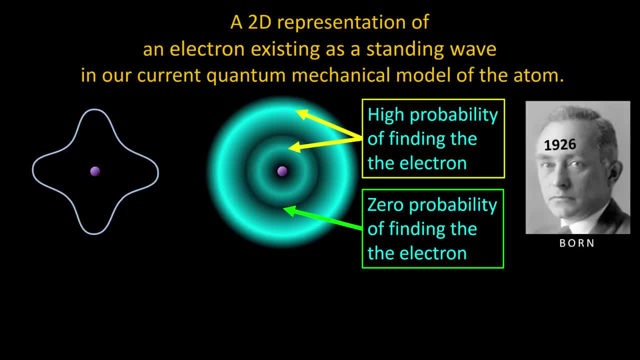 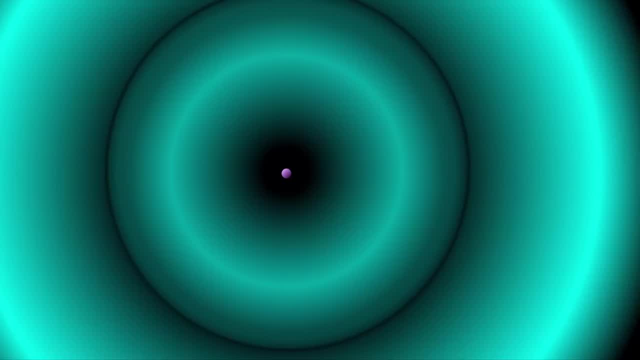 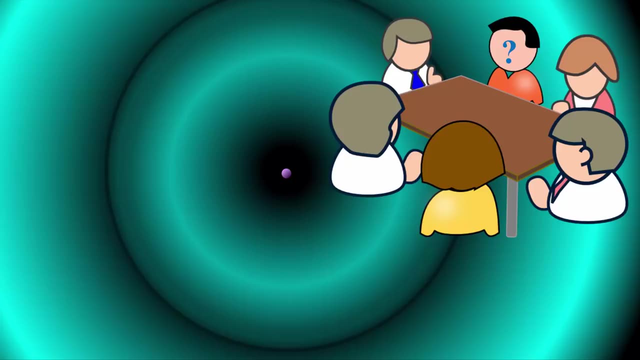 of the electron to represent the probability of where an electron is within the atom. One last fun bit about de Broglie: When he presented this work to his PhD students- the Mathematics Establishing Wave-Particle Duality- the committee could find no fault with the math. 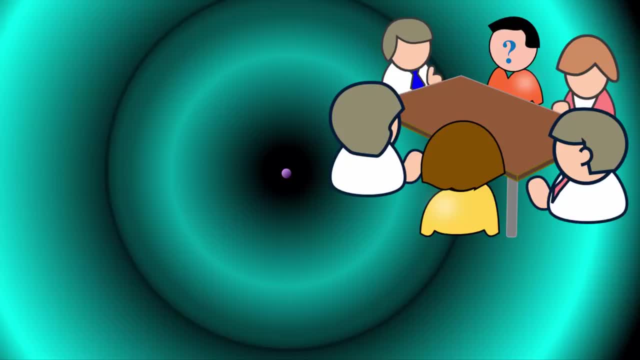 but they had great difficulty accepting an electron behaving as a wave. To help make their decision of whether to give de Broglie his PhD, they sent off de Broglie's dissertation to Einstein, who wrote back and told them that the idea had merit.